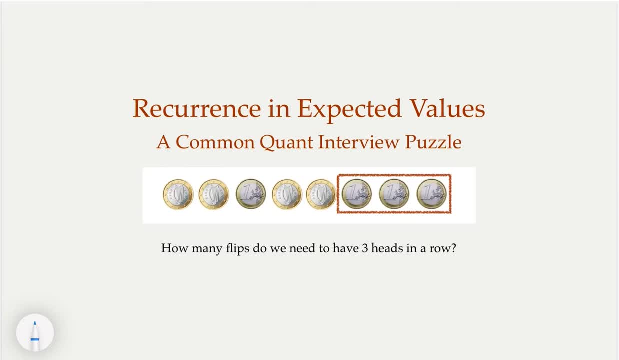 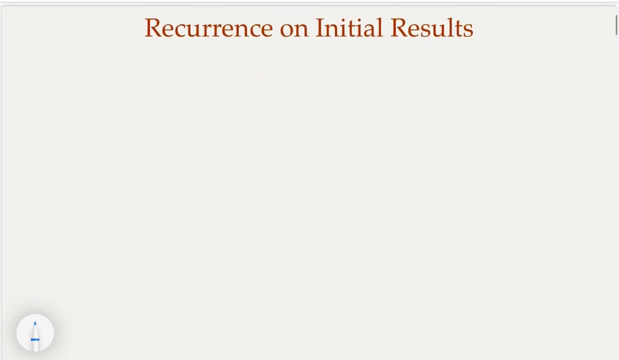 row. Alright, so today we're going to introduce some recurrence method in solving this problem. So in the first method we're going to do the recurrence on the initial results. You flip a coin. you could get a head or tail, So you get a head. good news, you get a chance to get three heads. right. But if 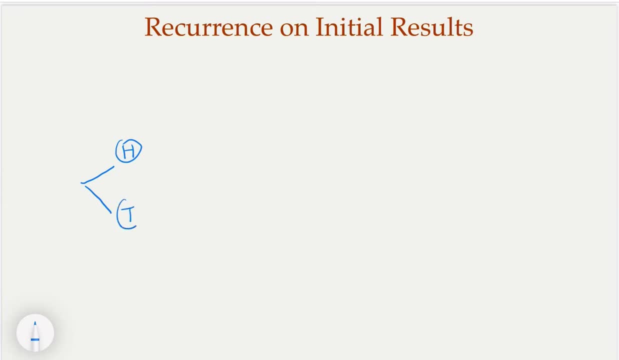 you get a tail, then you have to restart. So if we are looking for some unknown value, if you are a 2-star you have to restart. So the third method is going to value. we create X. what is X? X is number of runs to achieve H, H, H as the results. 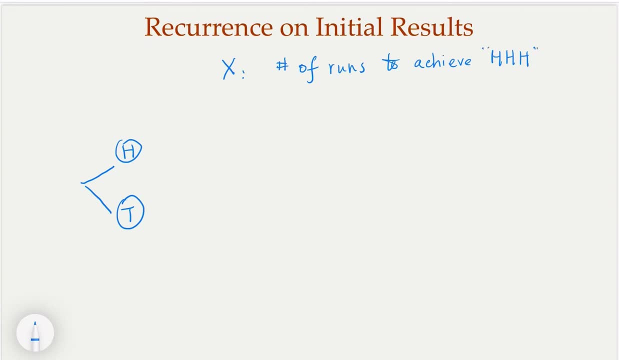 right. so this is a random variable. we try to see what is the expected value of that right. so if X is the expected value and you flip, you could tell you already waste the one flips and then on the every you still need X number of runs. so you would need, on the average- this is on the average. now what is? 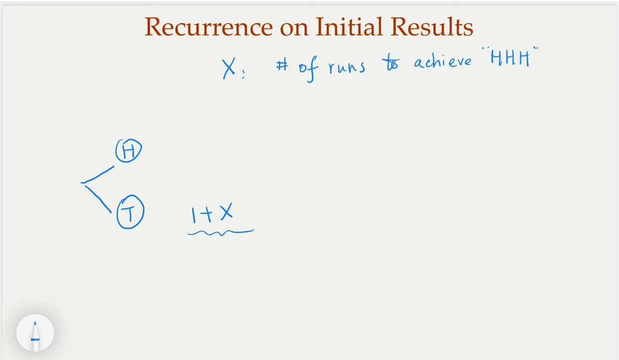 probability that even happening, that's one half of opportunity. so the probability here is one half for this to happen now. if you could edge, that's good news. but then you have the second flip in the second clip. you still have half and half chance, as is all have a chance, to get a hair or tail. if you could tell is even worse. 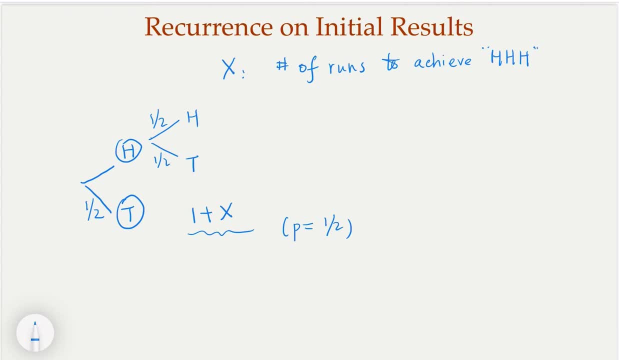 than the first result because you wasted two flips. so, in other words, on the average, you would need two plus X steps in order to get H, H, H, and the probability of this even happening is half times half, which is one quarters of chance right now in this case. that's good news. you have to edge and you see a hope. you flip. 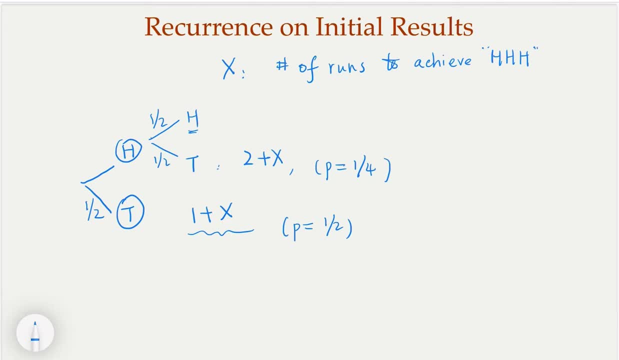 again the third one. if you get an edge, congratulations you get it, and how many steps you have done? three, and this, of course. this event happens with probability of one eighth right, and, of course, if you could tell how that's miserable, you wasted three steps, so which means, on the average, you would require another X steps in order. 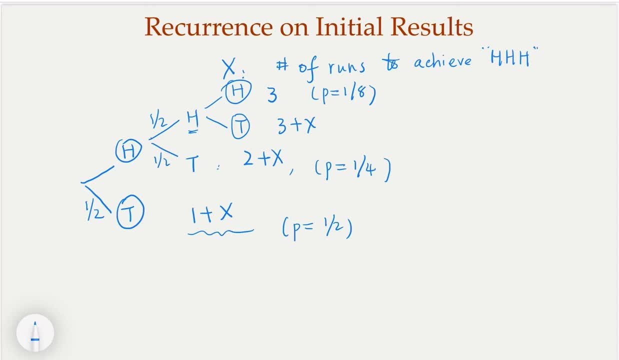 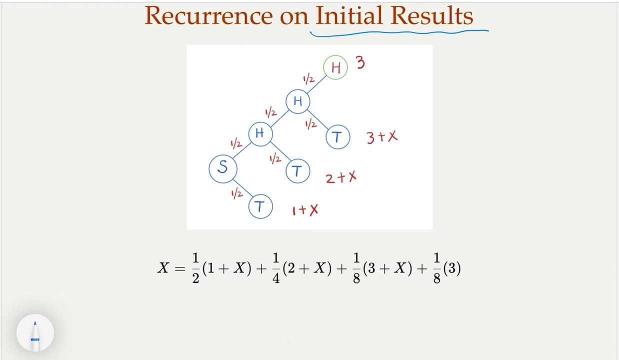 to get H, H, H. so with this event happens with one eighth of probability. so we this, we have a recurrence relationship. all right, let's recap. so here, depending on the initial results, right, initial, the first one, the second one, the third one, and then we have this unknown variable that's expected value. 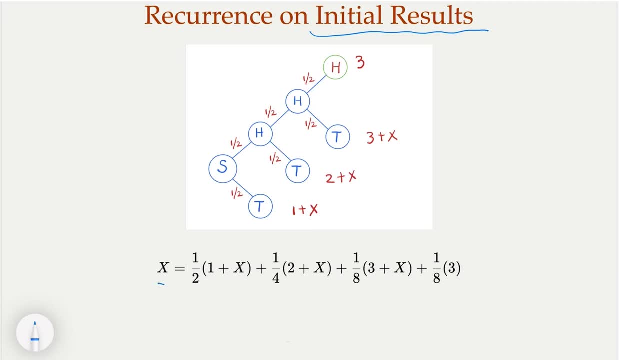 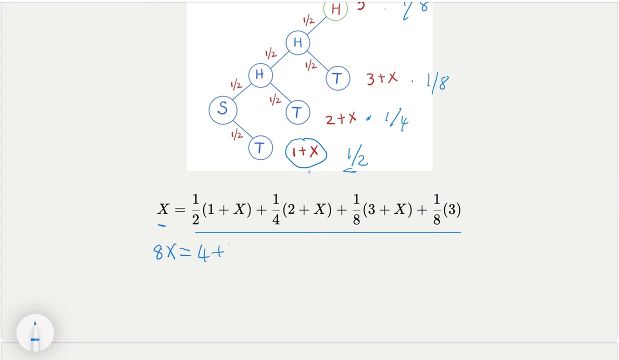 you know, satisfy this, this event, with different probabilities. one, you know, one half, and this one is one quarter. this one is one, is, and this one is also one is right. so you, you add it up. how to solve this linear equation? that's easy, you know. multiply it by eight. you got eight x equal four plus four, x plus four plus two x. 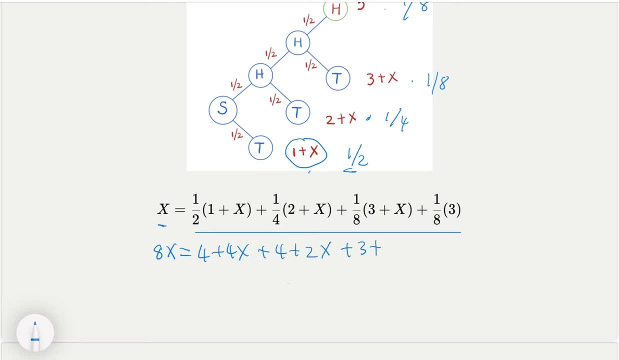 plus three plus x plus three, and then this would be seven: x. you get x here, and then four, four, three, three x equal fourteen. that's the answer. okay, in other words, by using the recurrence, we conclude that it takes about 14 steps in order to see: hhh, okay, with a fair coin, this is the method number. 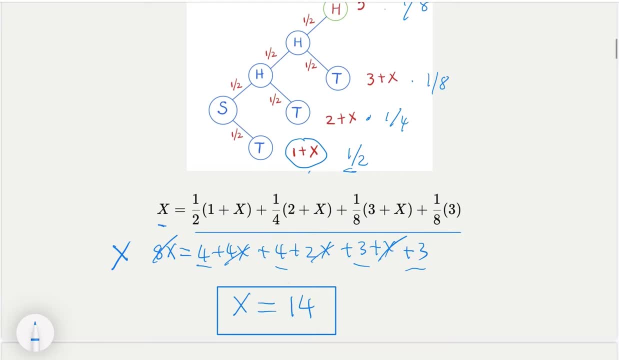 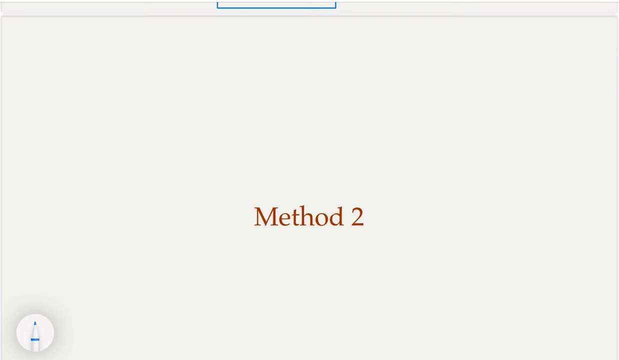 one, all right. on the method number two, we're gonna take a different approach now. think about it: in order to have- hhh, three h in a row, you must first have two h in a row. without that, you're going to start over, right? so if you have two h in a row and then you have another one, you get a chance, right. 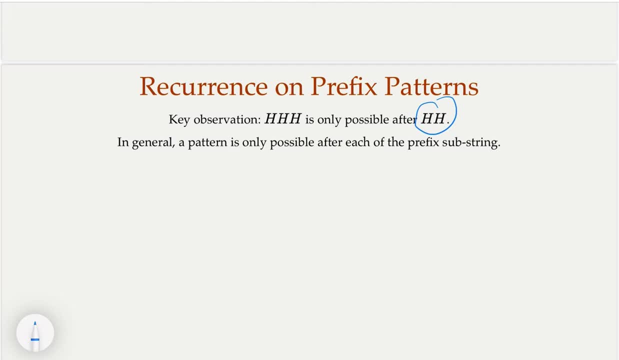 now. similarly, in order to achieve two h in a row, you must see the first edge first right. so, in other words, in any pattern you would like to see, in order for the pattern to happen, you need all the prefix substring to happen first right. so in, for example, if we're looking for 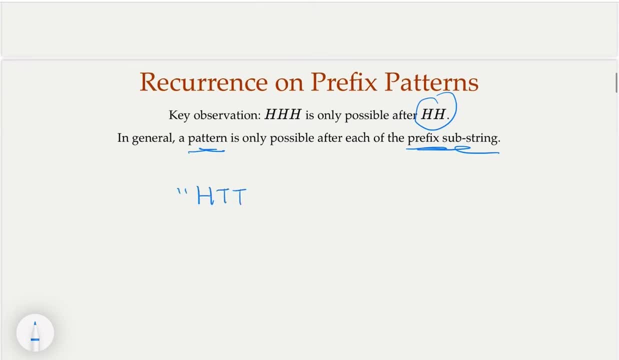 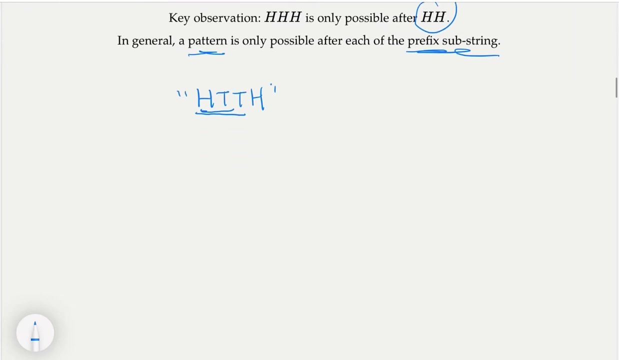 htth in order to see that, you have to see htd first. in order to see htt, you need to see ht first. in order to see ht, you need to see h first. all right, so we're gonna do recurrence on the prefix of the pattern. so here we're gonna say some notation. here we'll say ri- the average number of runs, in order to see. 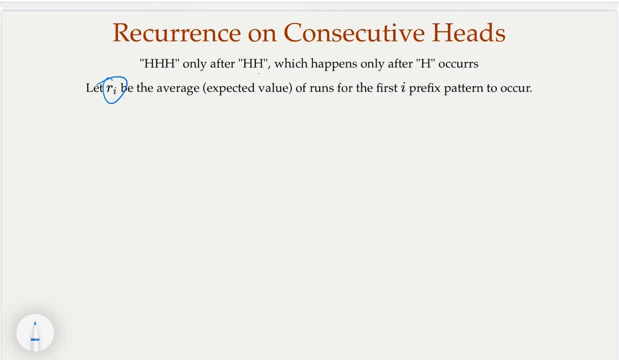 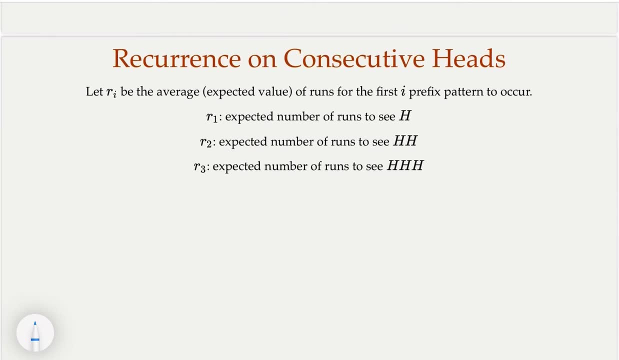 the first i prefix. in other words, here is the notation. in order to have three edge, you need to see one edge first. let r1 be the expected number of runs to see one edge now. similarly, r2 for 2h, r3. you can continue. you know, if you want to see 10 edge, that'll be r10. you know this would have. you know now what. 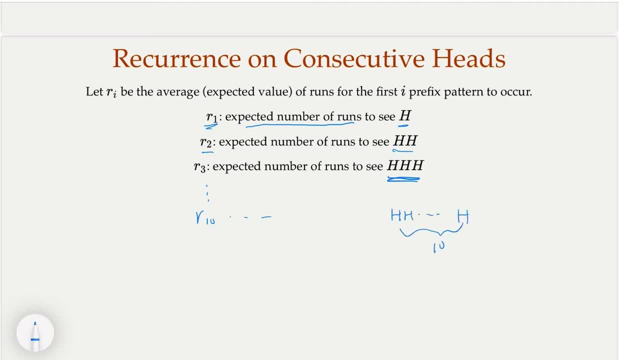 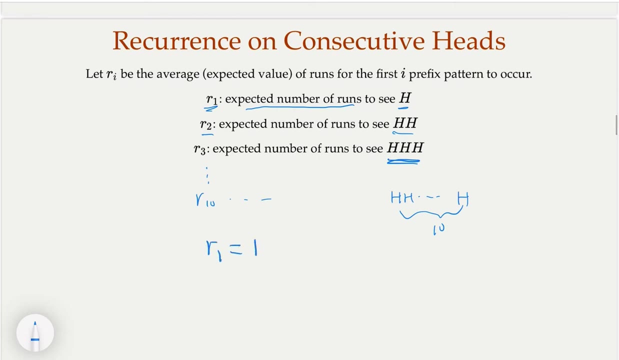 is recurrence relationship. let's think about it right. so for the first one, okay. so in order to have r1, of course you need to at least flip one time right, so r1 would equal one. you need to do that, you know, to see the results. now, if you have edge, you're good. 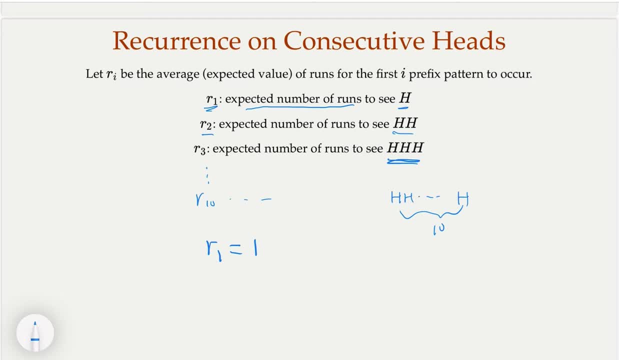 all right, you get a one edge, but if you get a tail with half of probability, then you on average you need another r1 steps. in other words, this one recurrence is like self recurrence, with the one half opportunity you could tell and then either take another r1 steps for you to see first edge now, similarly for our two. 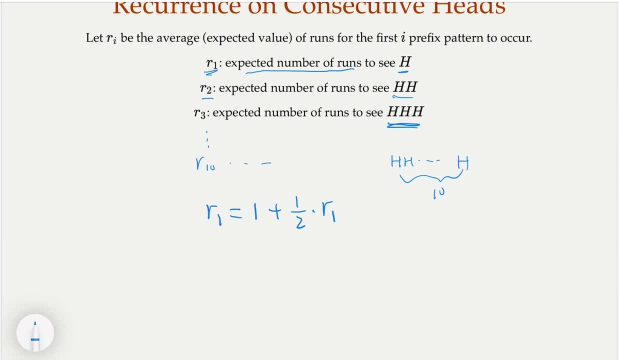 so r2 here. in order to have r2, you take on the average r1 to see one edge first. so you have r1 and then you have seen one edge. you need to have another flip, another unit plus one in this new results. if he is head, you're happy. but 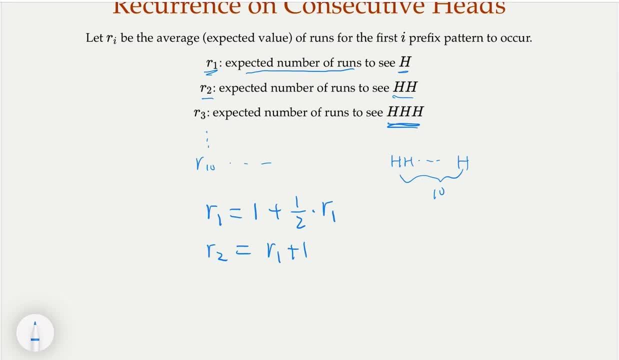 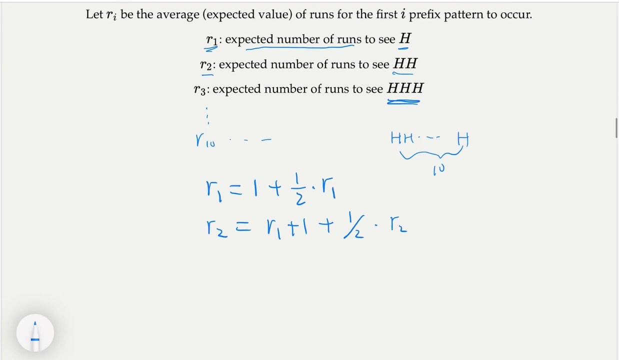 with half chance- you know half of probability- you're gonna see a tail. in that case, either require on average r2 to see two edge again. so the recurrence is that with one half times r2. now you can use similar arguments in that in order to see r3 you need to see two edge first on the average. it takes this much time right and 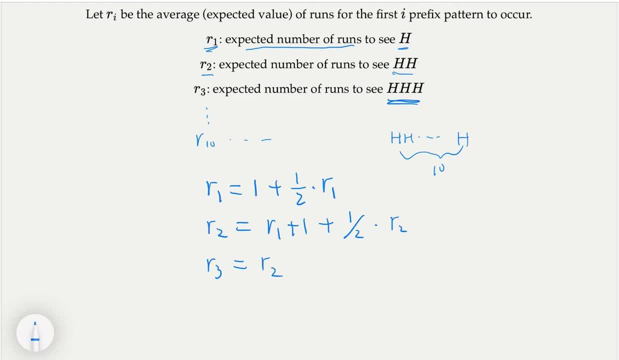 then you need to flip again. you hope to get three edge, so plus one. however, you could a tail with half chance, and then you need to flip again in a hope to get three edge, so plus one. however, you could a tail with half of opportunity, and then you need to start over again, so one half and then in. 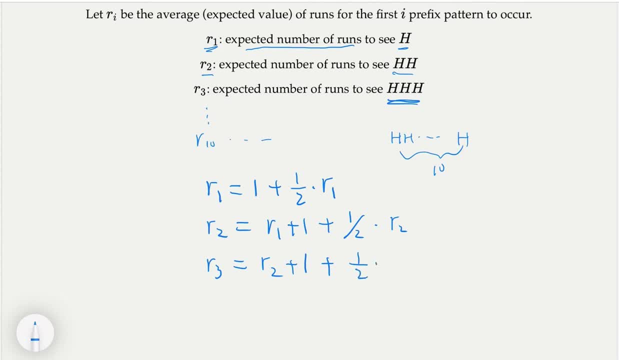 that case you need to take r3 steps in order to see three edge. all right, so that's good. so let's recap. so here, in this case, yeah, r1 has equal to two. right, that makes sense. right, it, on the average, is a fair coin on the average you have. 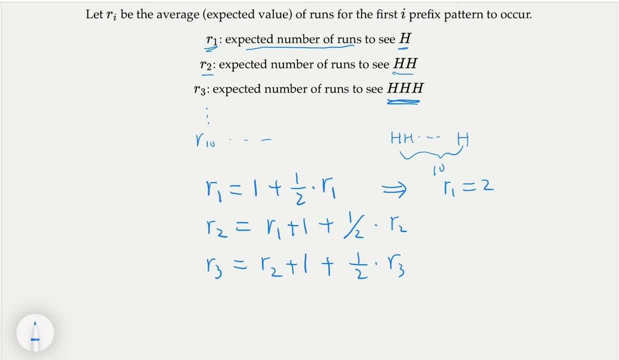 two tries in order to see one half now. now for this one. let's rewrite it right: so that is half of r2, equal r1 plus one. multiply two. here this will be two is going to be two. yeah, so similarly, you can continue in general, you're gonna have this recurrence, okay, so how do you? 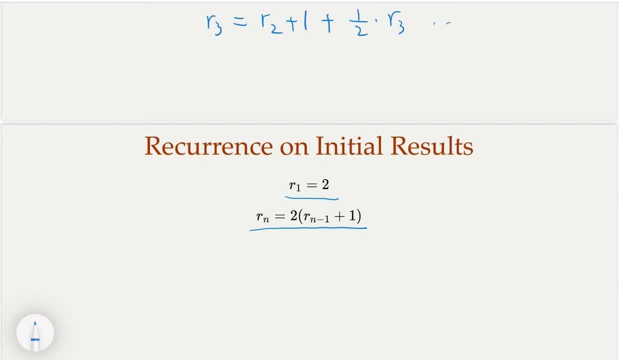 solve this sequence. that's easy. what you do is we change a little bit. you plus 2 on both sides, and then equal to our minus 1, plus 1 plus 2 and equal to plus 2. that's a geometric sequence, right? that's good. so the solution would be 23. 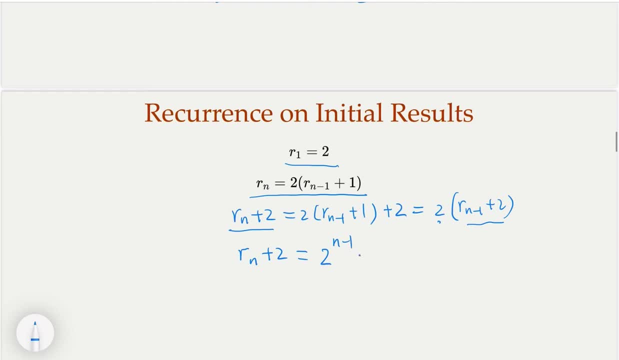 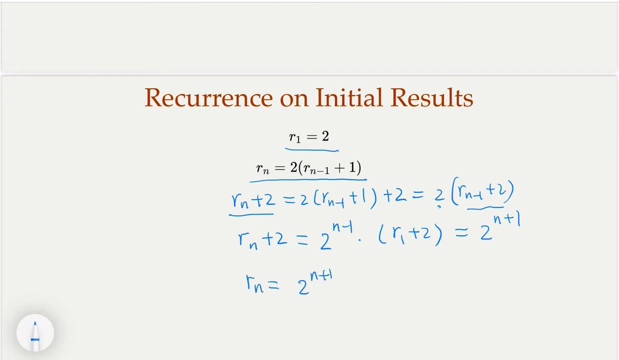 minus one minus two power times. the first term. first term is r1 plus 2. r1 is equal to 2, so that would be 2n plus 1. and then what is rn? rrn would equal to 2n plus 1 minus 2. in this case, we're looking for r3. 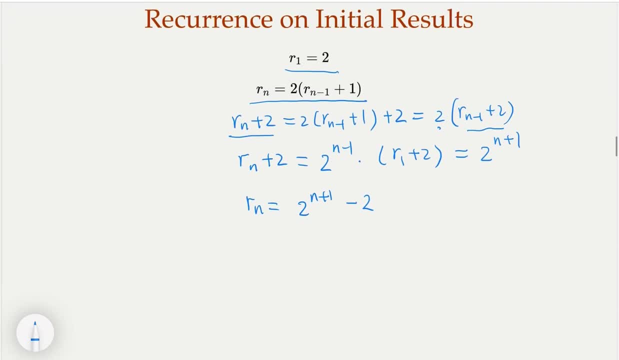 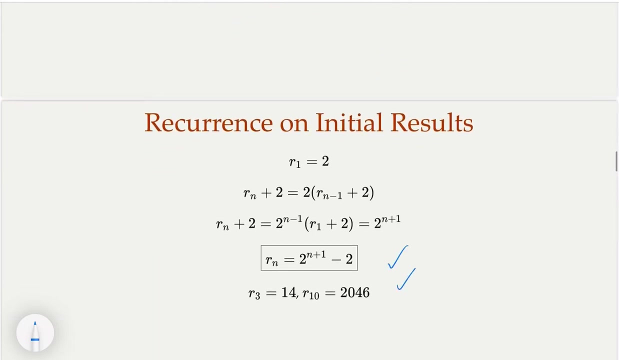 the number of runs in order to see: hhh. so plug that in r3 would equal 2 to the fourth power. minus 2, that's equal 14. same answer, all right, so that's good, that's what we have, okay. so as a reference, if you want to say 10 has in a row on the average, you need play. 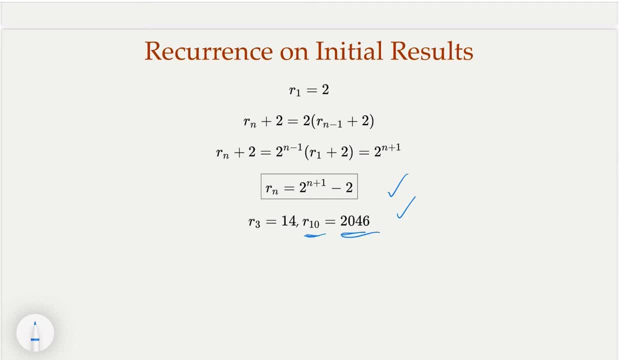 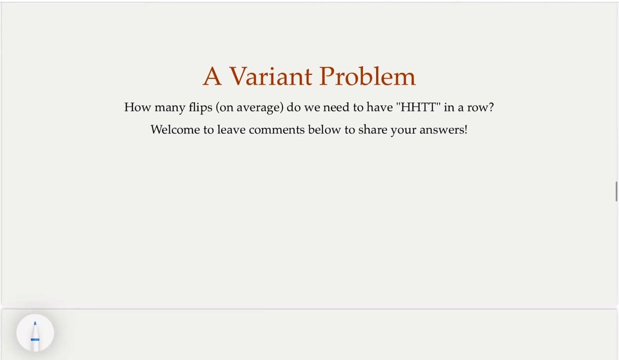 2 000 plus times. right, all right, that's good. that's for the second method. now for the third method. if you are familiar with what is called the um markov chain, you know we're going to cover that now. before we do that, i do have a variant of the. 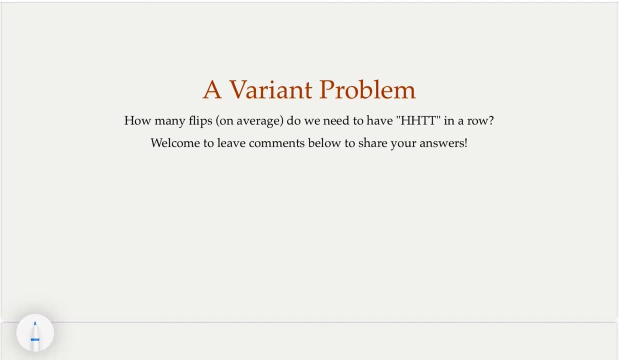 problem here if we're looking for different pattern rather than hhs, what if we want to see this hhtt? how would you do that? all right, so welcome to leave a comment below to share your answers. right, and i think you probably can use this second method here to get an answer. all right? 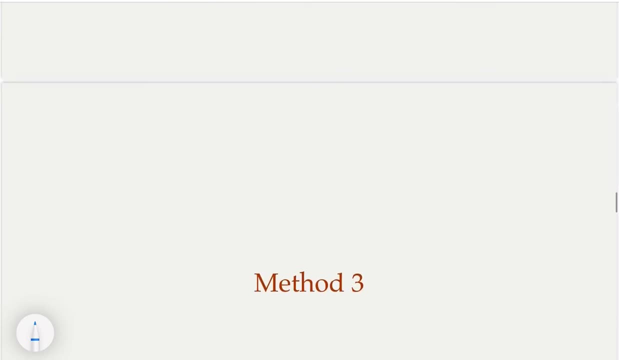 so let's come to the third one. as i mentioned earlier, is the recurrence with markov chain. now, for those of you who are not familiar with this concept, you probably either stop this video or do some research about it. so markov chain: sometimes very easy to model certain events. 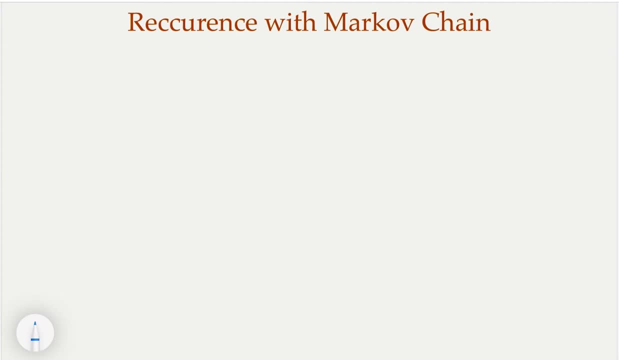 where i have a different state and there's different, you know, transitional properties from one state to the next state and also this key property that each state- the current state and then the state of the next state- you know only depends on the current state, does not depend on. 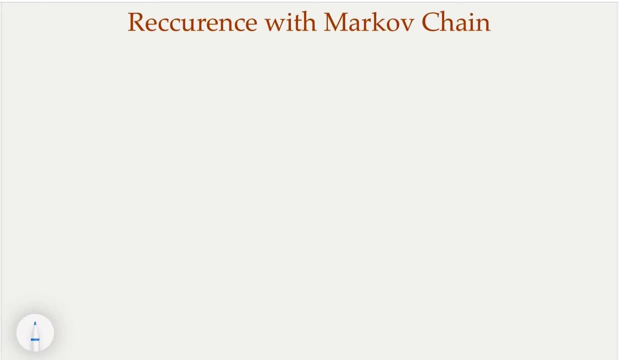 history of it, you know. in other words, conditional probability of your next step, next state, only depends on your current state, not the history. it's called memoryless property of markov chain or markov process, you know. so it's a very powerful tool in probability. but if you have not learned, 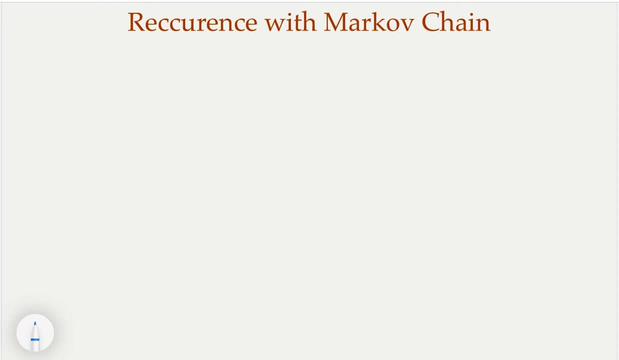 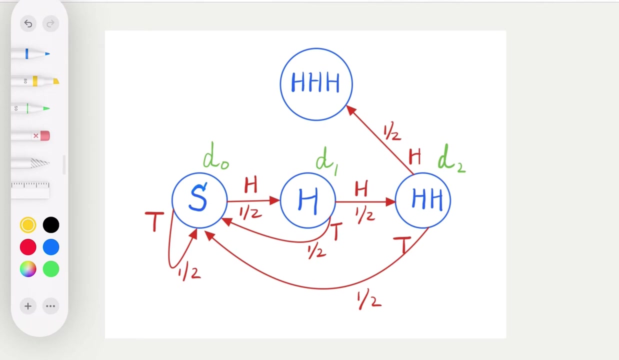 that that's okay. all right, but if you do, let's try that. so here the idea that we're going to model the event with the initial state, right, the initial state at the start of the game and then later you have a different transition function here and with this, like if you get a head, you're going to go to the state where there's one edge. 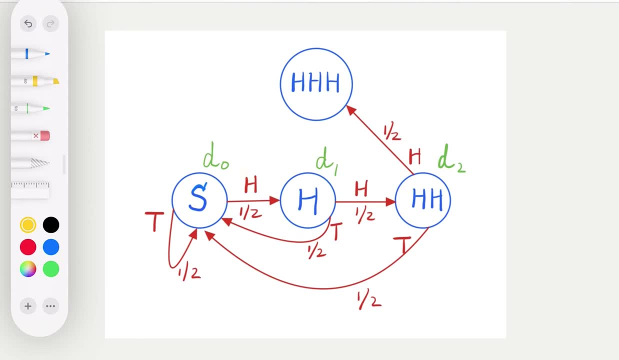 right. if you have another edge, then you go to next state, and then, if another edge, you go to the final state. this is the happy state. this is where, and you know we- this is what we want. however, in every state, for example, if you got a tail, you're going to go back to the, to the. 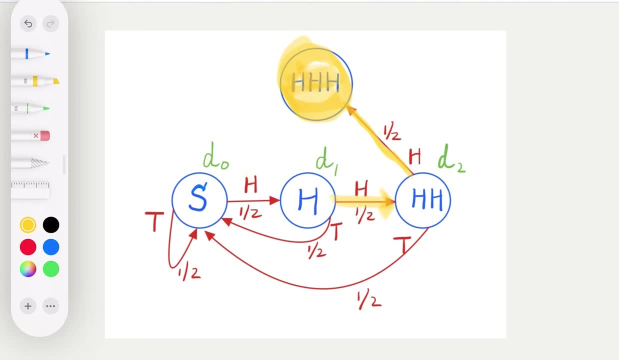 original one here, because if you get a tail, you you're going to restart, right, because you are looking for hh, right. so if you got a tail here and you know you're going to go back right. so that's kind of a state transition diagram and the number here would be the state transition diagram. 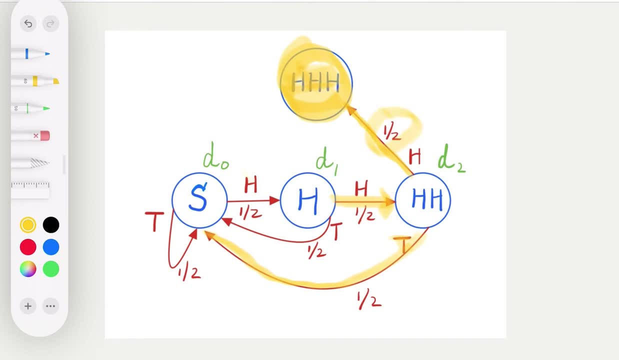 what is the probability from one state to the other state here? because the coin is fair, so each time it will have half a chance to get head and tail and you transition to different states accordingly, and also it's a memory list. Notice that, whatever happens. 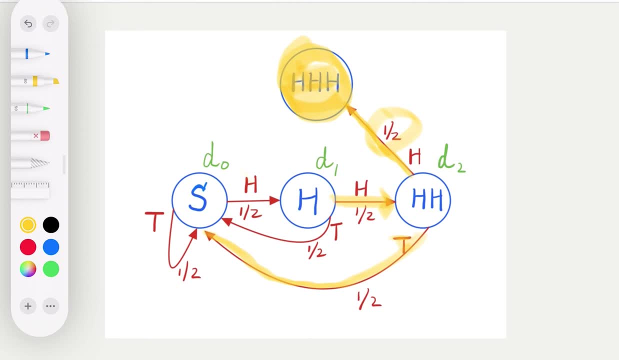 doesn't really depend on your history of it, right? It doesn't matter how many steps you have gone through to reach the starting state, right? It only depends on the current state, and then if you get edge versus tail in this case, okay. 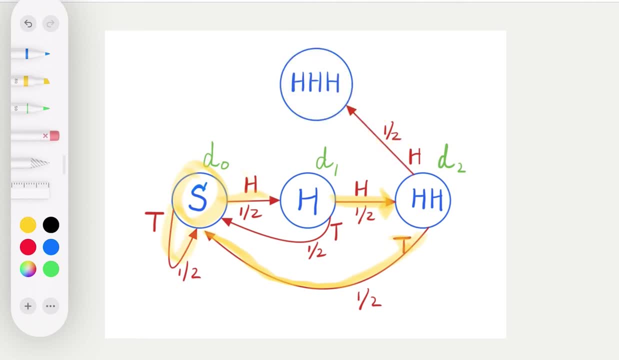 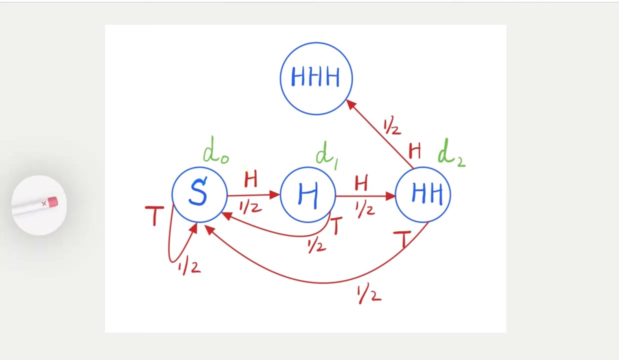 I'm going to erase all that. So here, with this Markov chain model of our game, we're going to have recurrence on what is called the D here. What is the D here? This is the number of steps you have to go through. 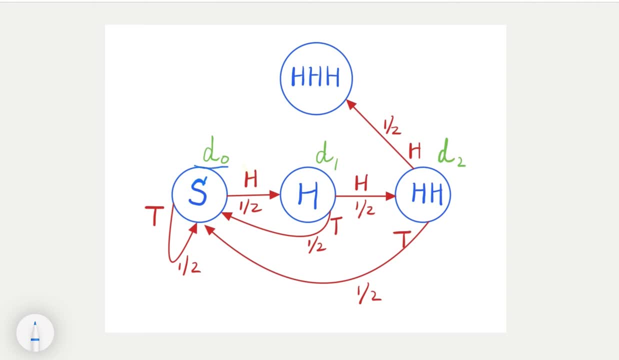 in order to reach the final good state or the accept state. This is the accept state or terminating state, right. So here you take D0, here we're going to D1 and D2.. Now, of course, the number of steps we're going to interest in. 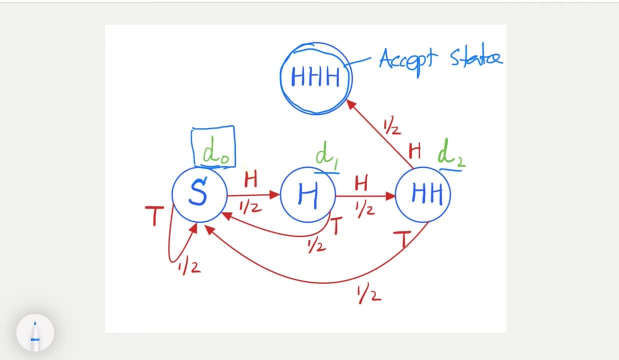 is what is D0 here? So what is the recurrence? So notice that let's figure out the D right. So each time, this is your ending goal right. So you want to get an edge, You're going to proceed. 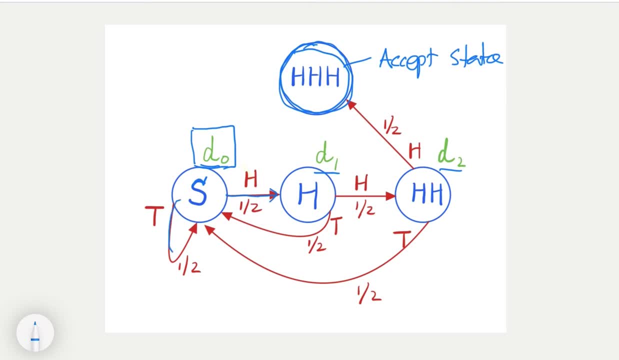 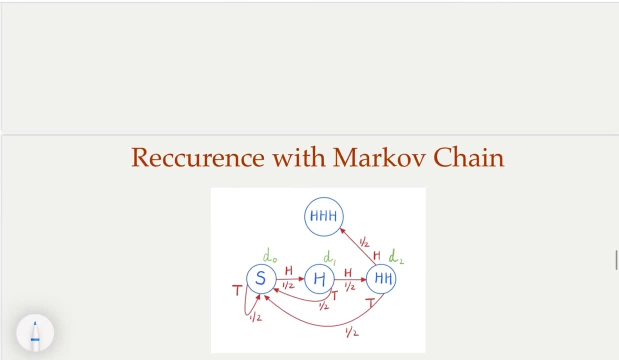 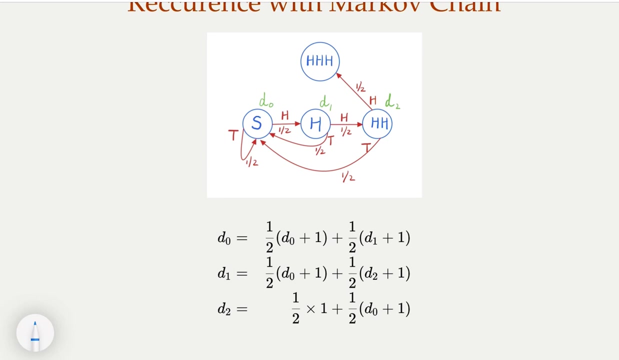 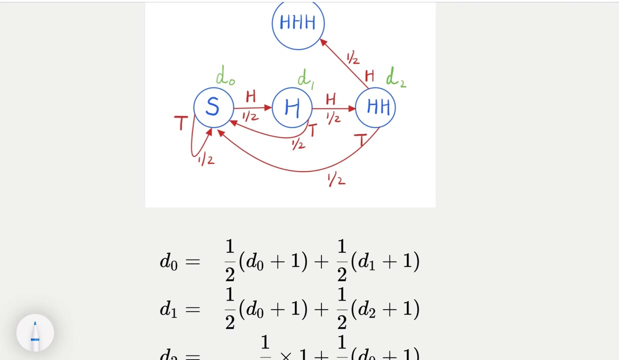 If you got a T, you know you have to restart. So with that, let's do the recurrence here. Yeah, I claim this is the recurrence. Let me explain why. that is the case For the first equation here. so you have half of opportunity to get a tail. 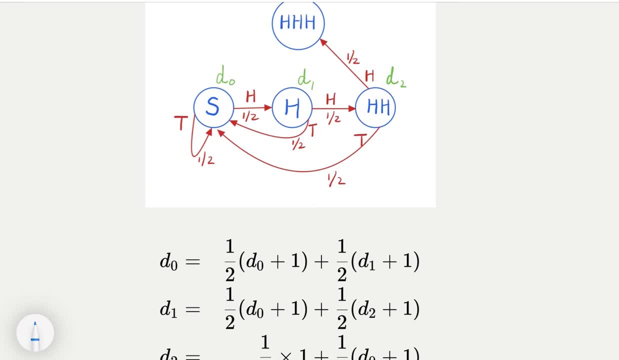 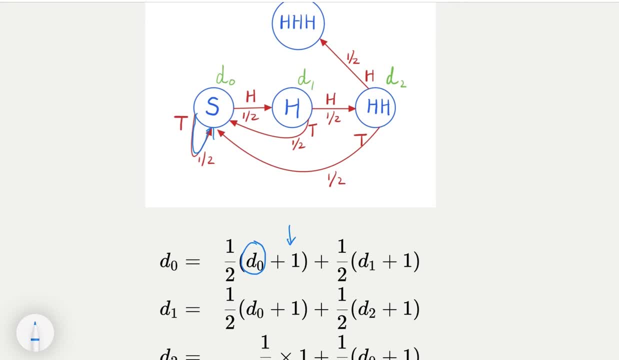 with the current steps right, You already wasted one flip, but you get a tail right with half of opportunity. But if you advance to the next state you got an edge with a half of opportunity. here you would require D1 plus 1,. 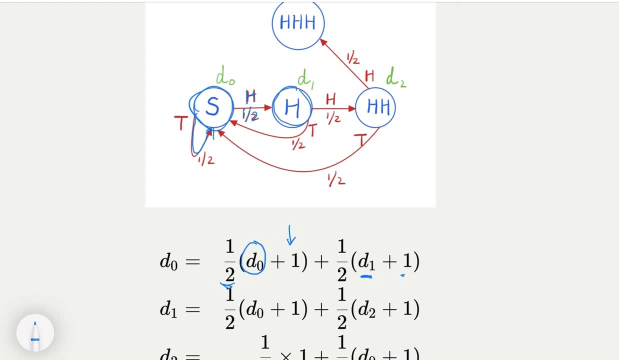 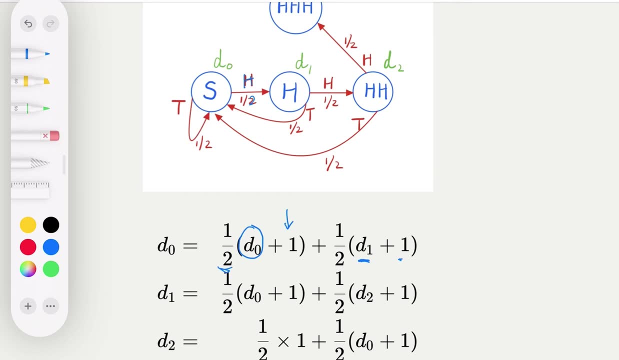 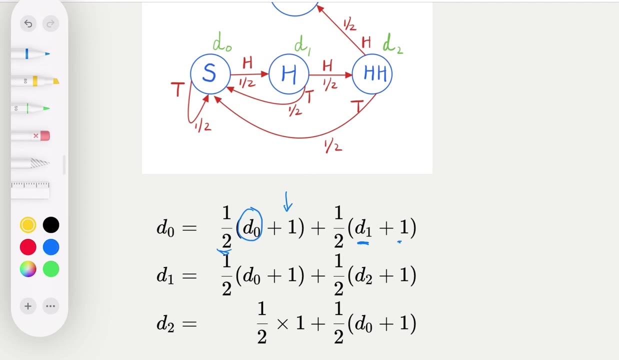 because you already flipped once right And then in that state it will take D1. first equation here: yeah, now the second equation is recurrence on the d1. so on the d1, here we're saying that you could go back. if you go to tail, you go back. 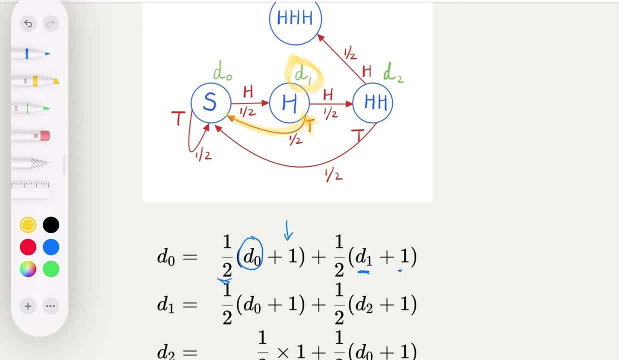 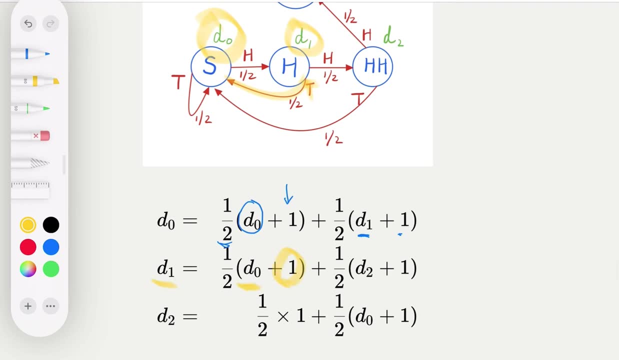 and then you go here. unfortunately, you take another d0 steps. so for the d1 you're gonna waste one step and then d0. but if you advance to d2, that's good right, so you're gonna put d2 plus one. yeah so, but if you are at a d2 here, 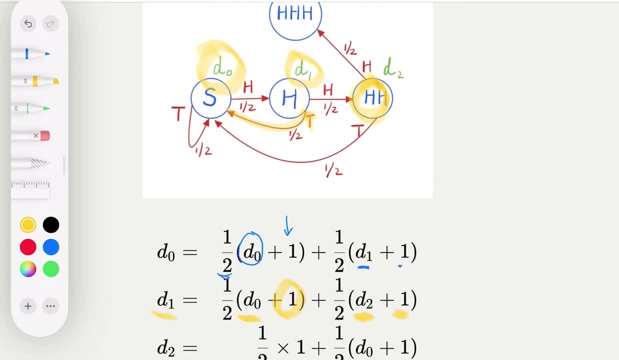 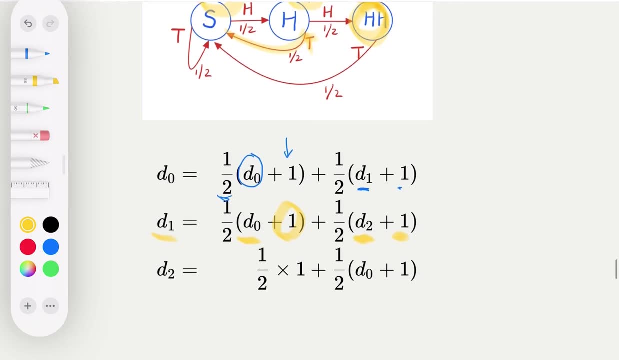 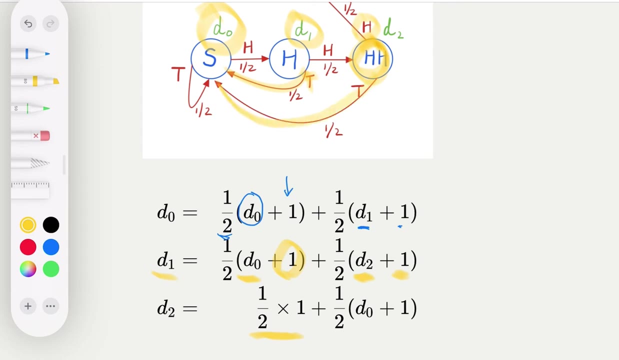 that's a d2 here and it require, you know, one steps. if you get an edge to reach the final state, so is equal half times one. or if you, unfortunately, you go back, right, you go back to d0, you go back to the starting state where you would. 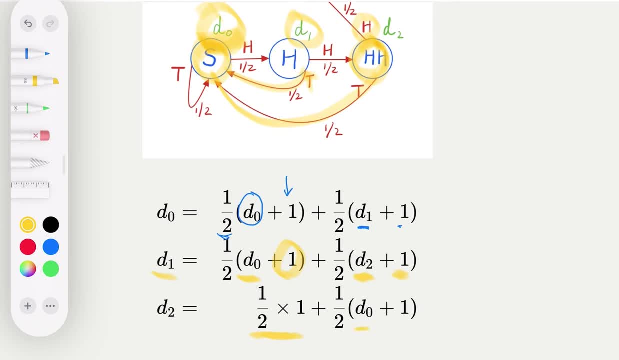 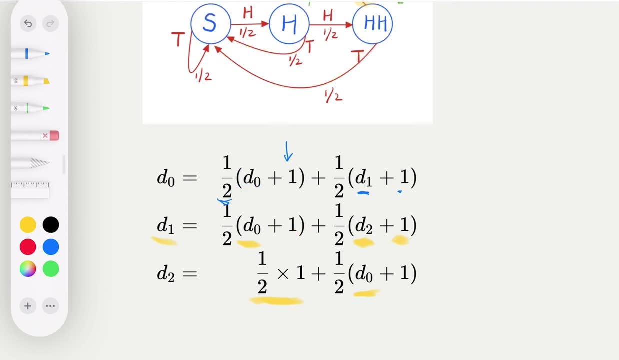 require d0 to reach the final goal, right. so there you go, and then you go back to the starting state where you would require d0 to reach the final goal, right? so there is a recurrence and the results is okay. so this recurrence exist, and how do you? 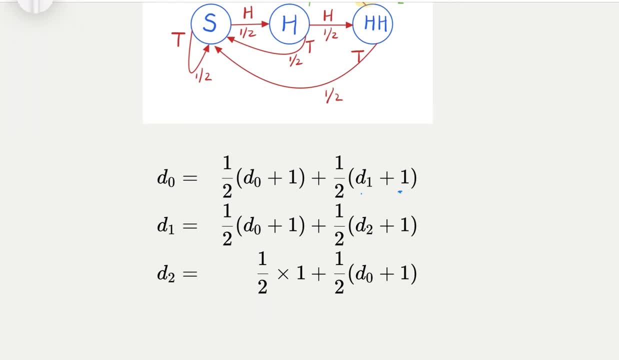 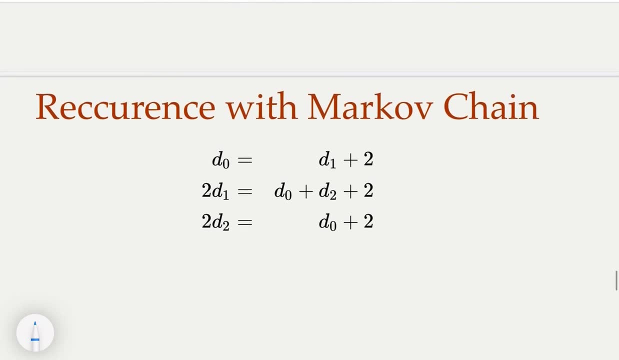 solve. we want to solve for d0. we don't care d1 or d2, right, so let's rewrite the equation here. this would be equation. and you want to solve for d0? right, so that's easy. you plug in d1 to here, right, so it'll be. 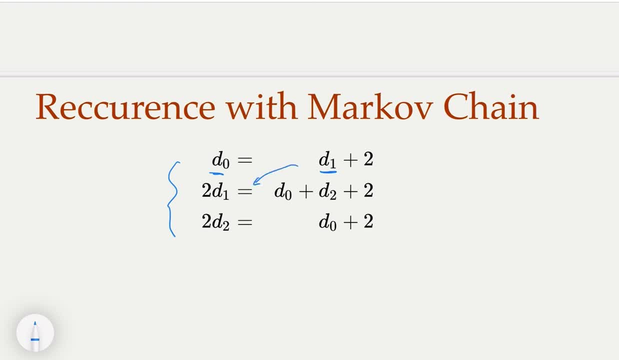 comes um 2d1. yeah, so 2 that would be 4, that would be 2: 0, so 2d1 would equal to 2d0 minus 4. yeah, equal d0. we want to replace d2. what is the d2? d2 is here half. d2 would be half of that right. 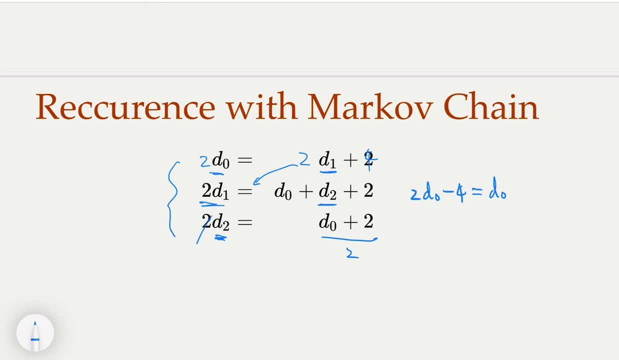 so plus half of d0, plus 2, yeah, and then plus 2, yeah. this is just the equation for d0, just solve it right. so multiply 2 on both sides. you got 4 minus 8, 2d0. this would be 4, right? so that would. 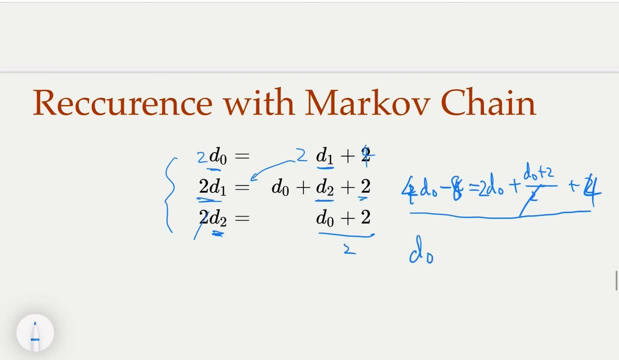 be d0, yeah, equal 8 plus 2 plus 4, equal 14. same answer. all right, good, so it's consistent with the other two methods, but this one we're going to model the problem with a markov chain and then we're going to define. 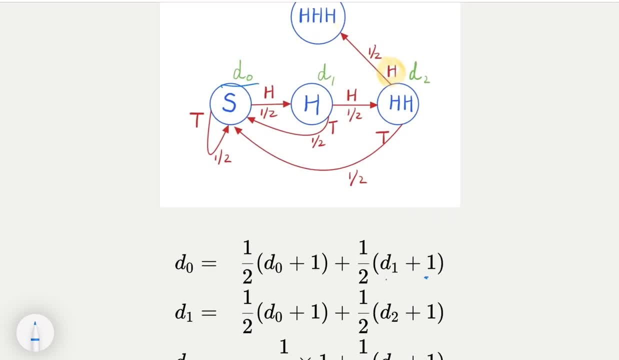 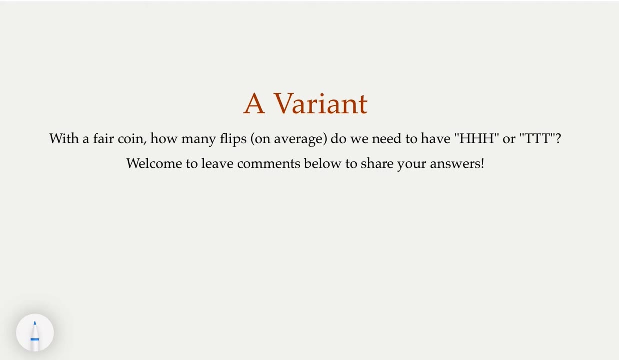 the recurrence on those three numbers. right, so that's good, all right. so i think this is a interesting problem. but let's raise another variant of the problem. that is, you still, we are dealing with fair coin, but here we're looking for either hhh or ttt. so how many? 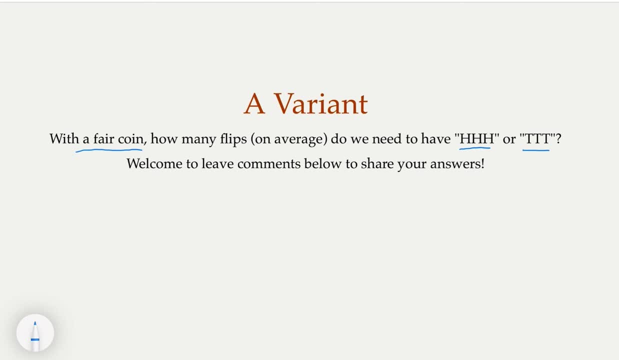 flips on the average do we need in order to see either hhh or ttt? okay, again, welcome to leave comments below and share your answers all right. so i'm curious to see how would you approach to solve this problem all right now. before you do that, i would like to share maybe another approach to answer this question. 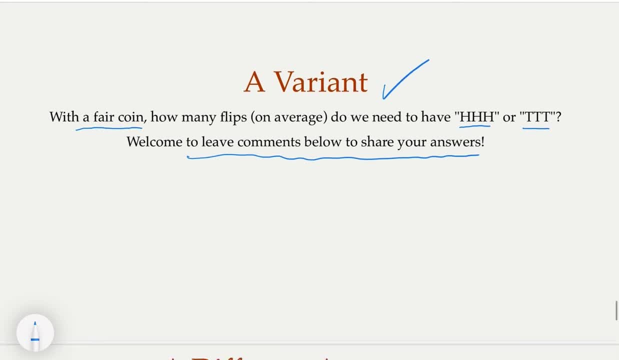 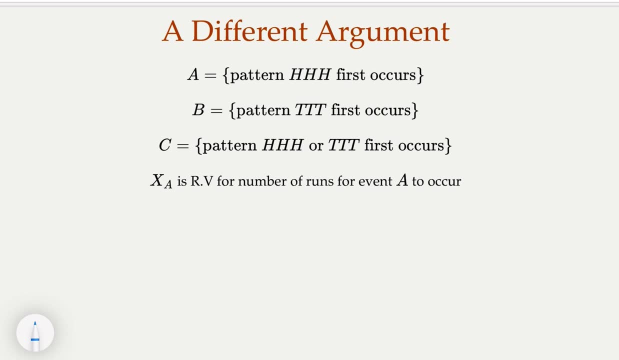 so here's another line of reasoning here. so let's say that even a is hhh first occurs, even the b is pattern, ttt first occurs and c would be pattern either, or we're interested in this, yeah. so notice that we already know the answer right. for even a, what is xa? 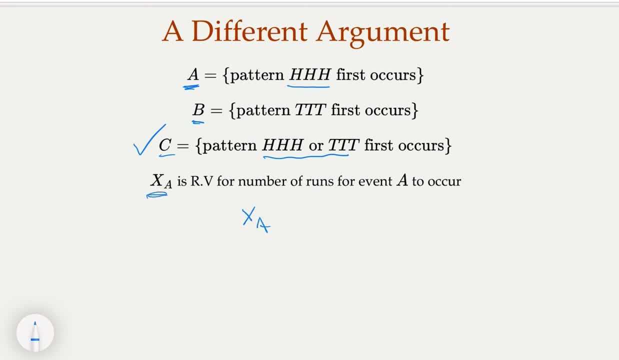 is a random variable for number of runs in order for a to first occur. so the expected value of this it would equal to 14, right? we solved it earlier now with tttf by, because it's symmetrical, right? so head, head, head and tattletail, they're the same thing, right? so we're going to solve this. 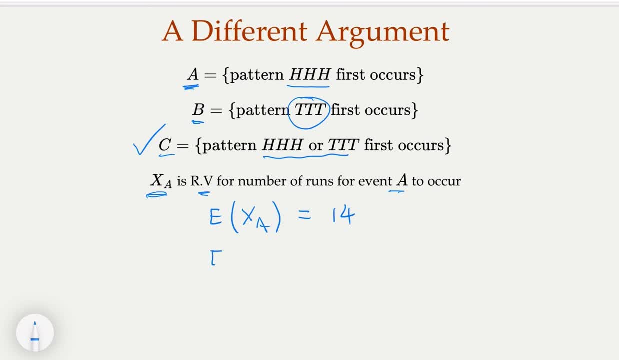 right, so you would know that the event xb would also equal to 14.. yeah, so think about it. what does it mean? so it means, on the average, every 14 steps, you're going to see hhh once, yeah, because the game stops once. you see that now, in the meantime, every 14 steps, on the average, you're going to see ttt. 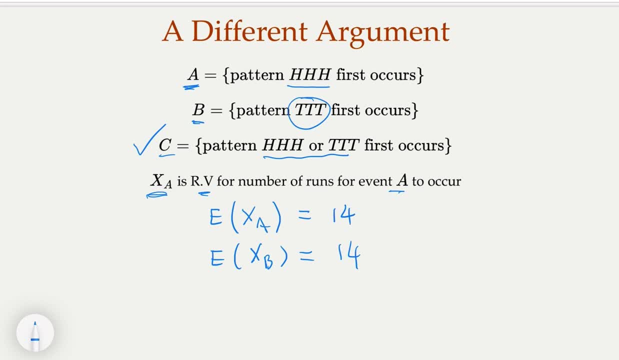 so, in other words, when you think about it on the average, every 14 steps you're going to see one ttt and one hhh. so for the event c, you're going to occurring twice on the average. again on the average. so which means we conclude that the expected value for xc equal to seven. yeah, 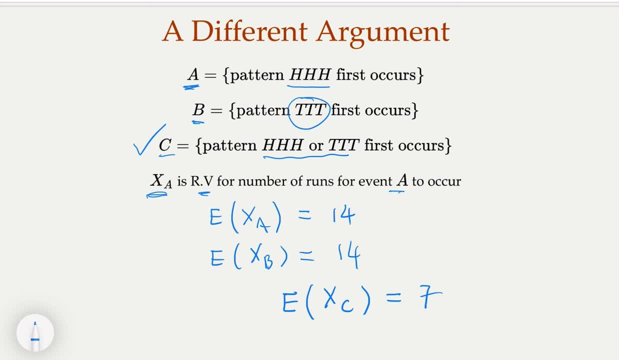 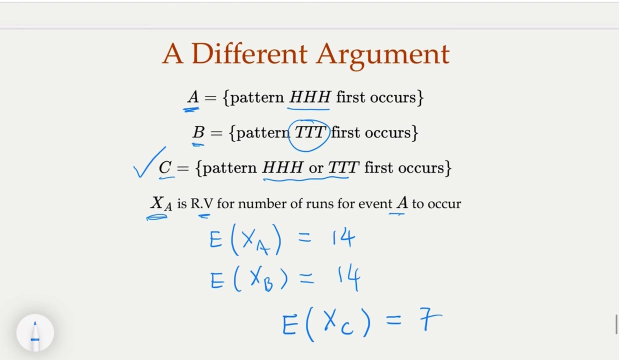 because, on the average, you're going to see two instance of that event for every 14 steps. all right, so the number of flips in order for us to see hhh or ttt is seven, or now, in this case, of course, and earlier we have this. uh, and let me see the for the consecutive.